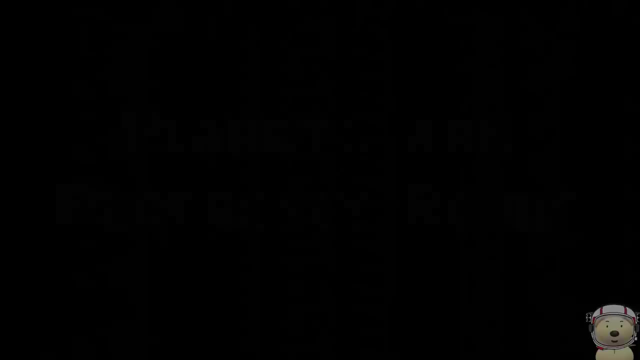 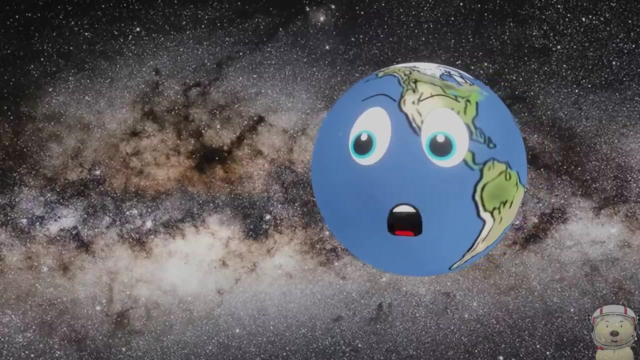 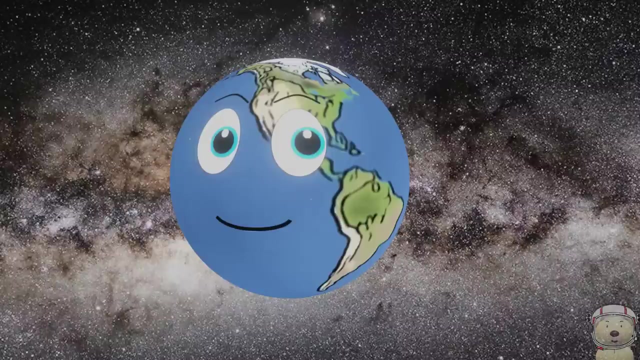 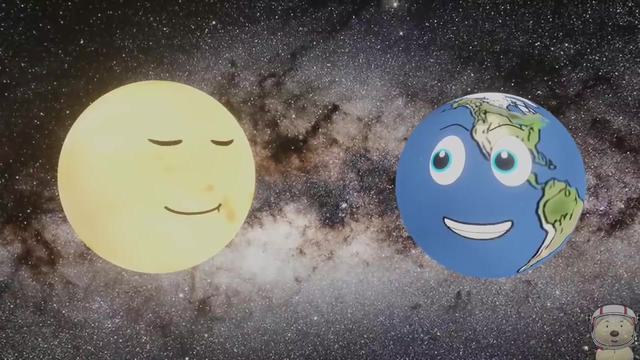 Yes, I am Wait there, Venus. Planets are perfectly round. Some people think that our planets are like a ball and are perfectly round. Wrong What? But I am perfectly round. Well, actually, Venus. yes you are. You are probably one of the most roundest of planets. 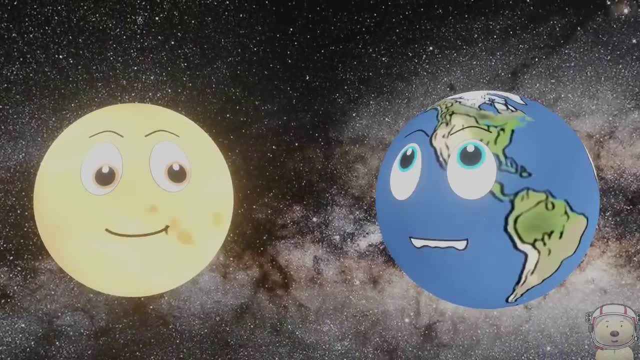 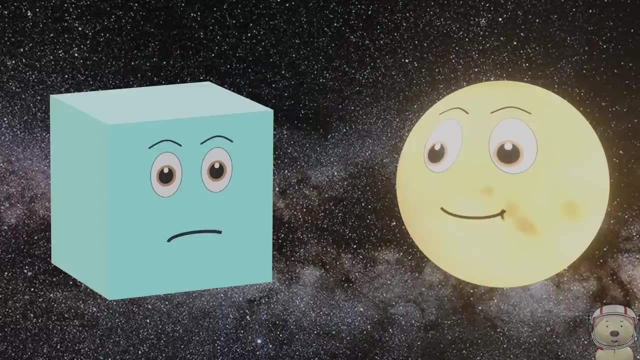 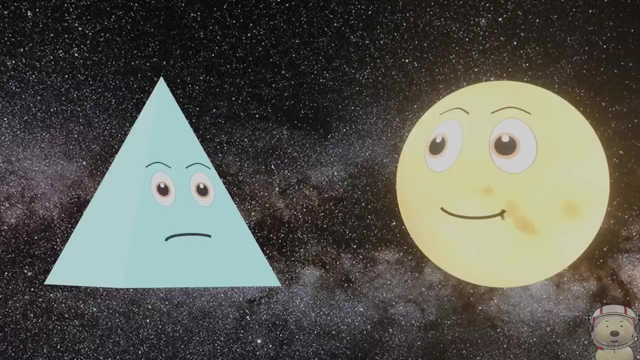 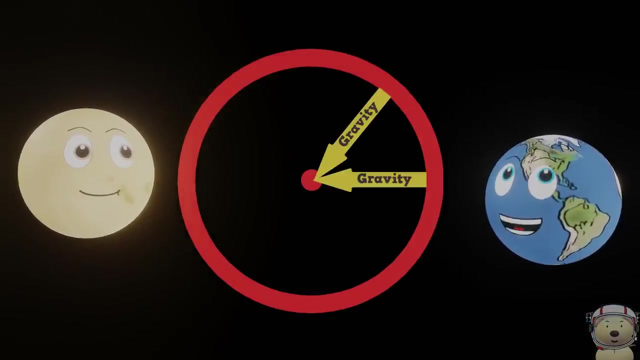 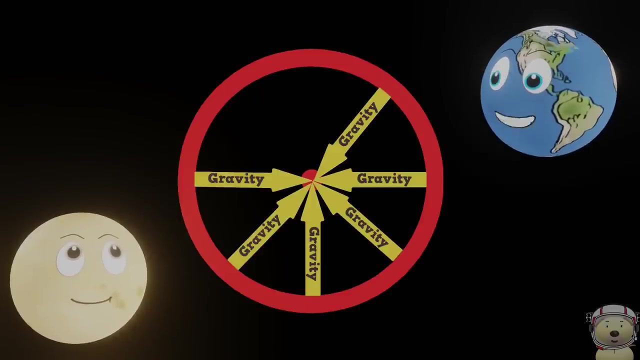 Perfect, you might say, Hmm, well, So why are planets shaped like a cube- Wait what? Or a pyramid? Stop that. A planet is round because of gravity. A planet's gravity pulls equally from all sides Because gravity pulls from the centre. this makes a sphere shape. 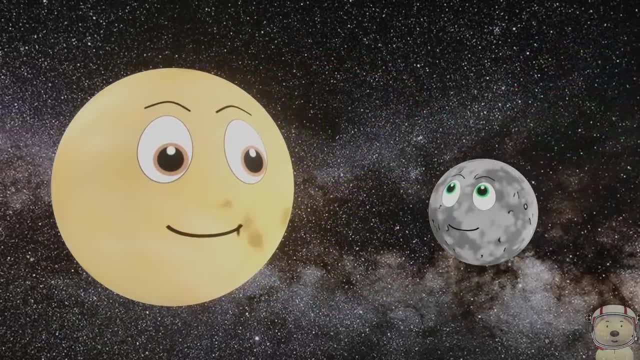 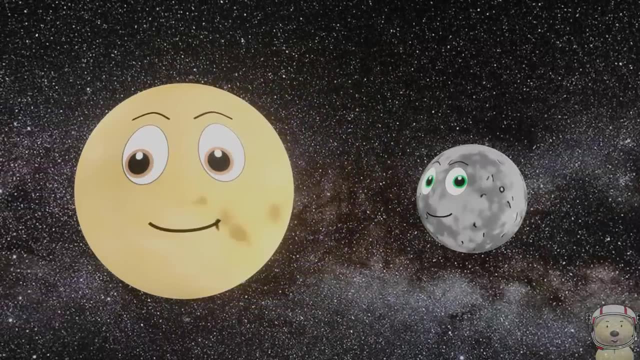 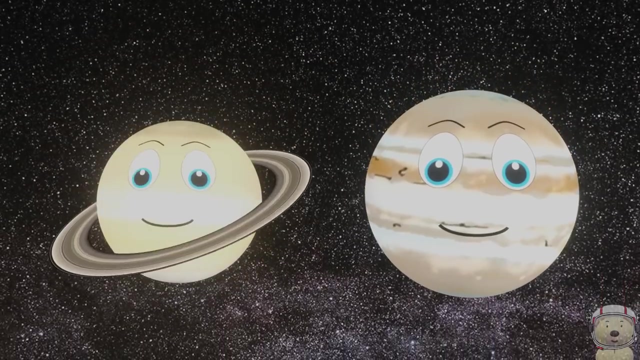 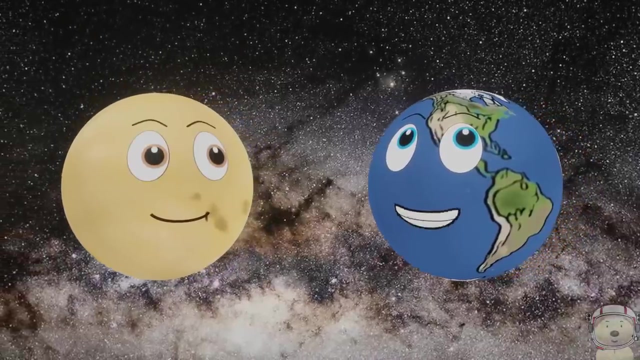 Ah, You and Mercury are the most round of all planets Because you spin so slowly. Who is the least round? Planets like Saturn and Jupiter actually bulge more in the middle Because they are so big and spin so fast. The other planets are between you and Saturn in Uranus. 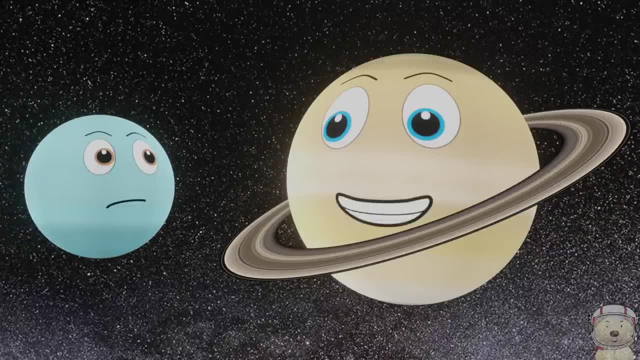 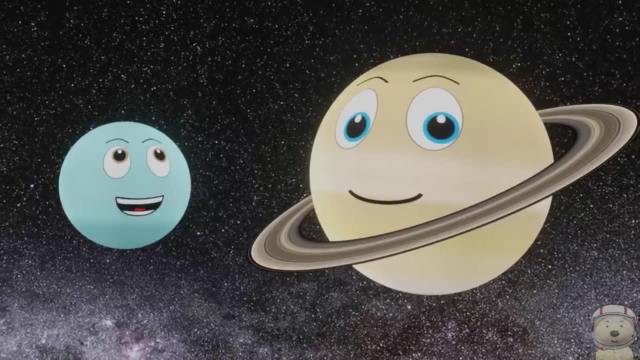 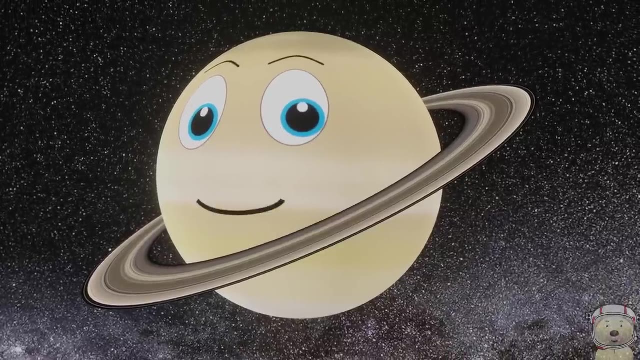 Hey Saturn, Hi Uranus dude, I've decided to re-sing the lyrics to Israel, The theme song. I don't think Neptune sings it right at all. Ah, Okay, Uranus dude, Let's hear it then, Is it? is it wrong? is it wrong now? 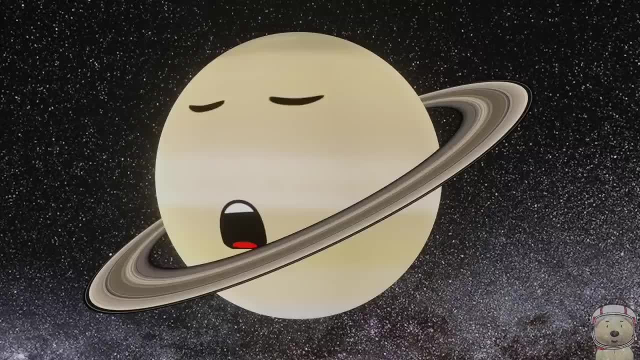 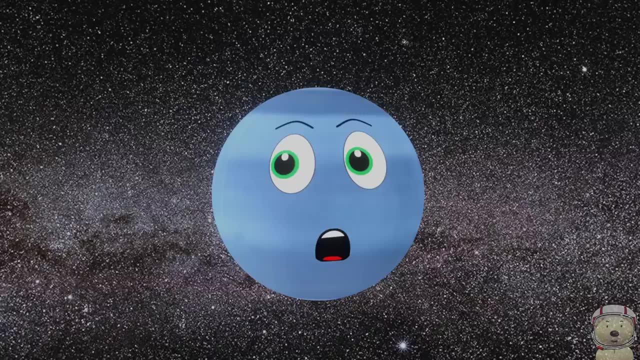 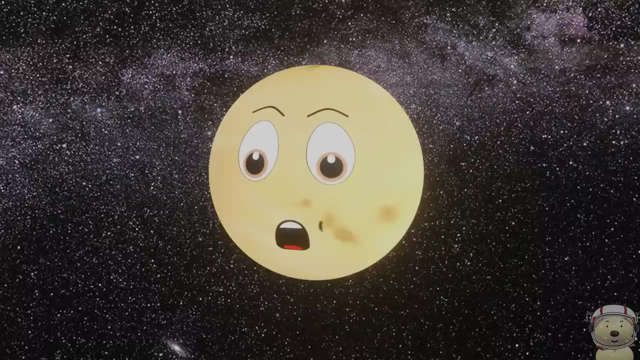 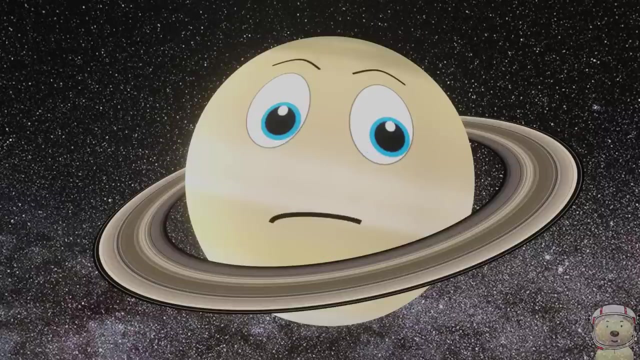 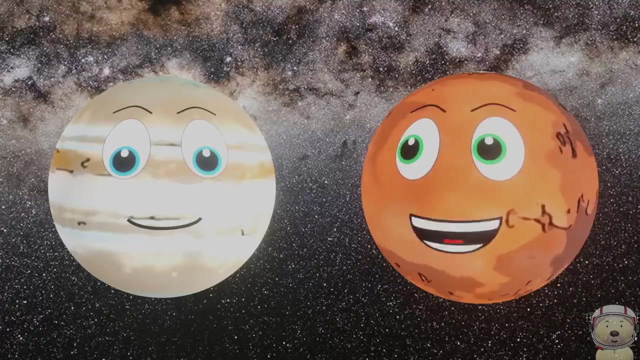 Tell me why you know it's wrong. Is it wrong? is it? is it wrong? Is it wrong now? Well, Uhhhh, Now one false fact that we have found: The planets are perfectly round. Bulge in the middle makes them look wide. 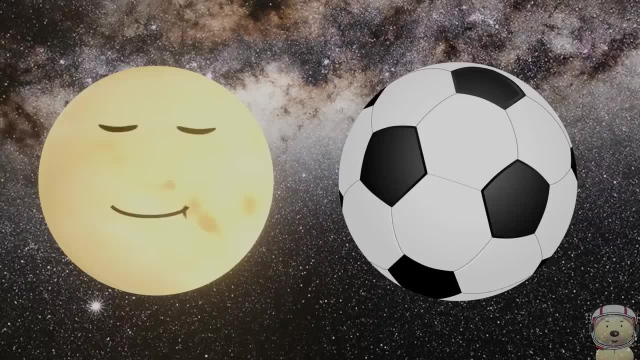 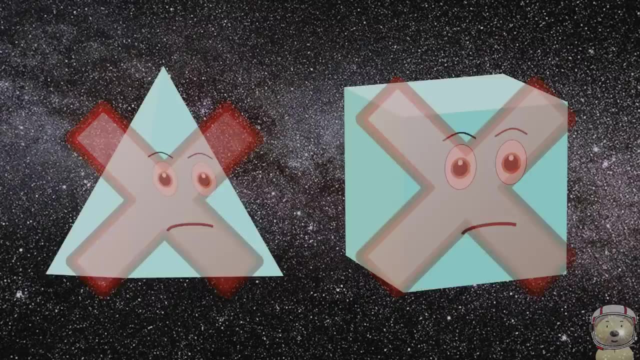 Toy Time Town. fact is denied. Planet Phoenix- Planet Phoenix is the most likeable, It is true. she's rounder than you all. Not like a pyramid, Not like a cube. Planet Mars, Rapping on YouTube, Oh yeah.